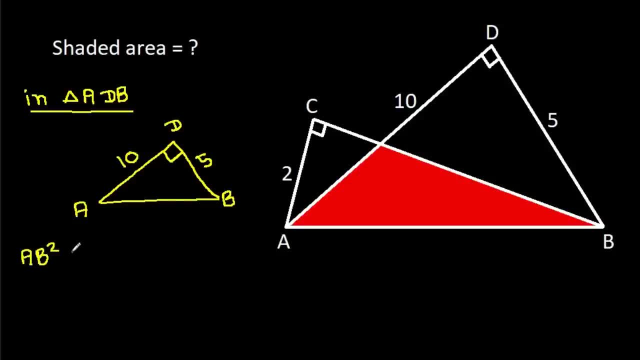 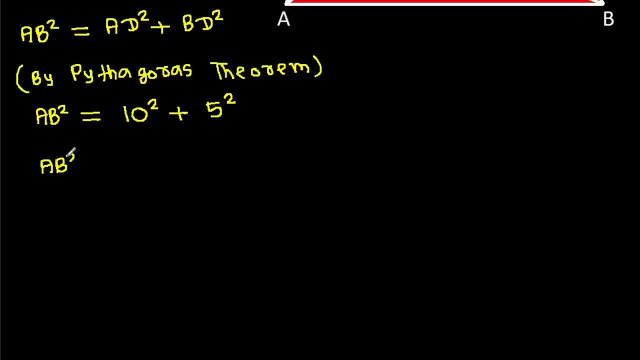 So ABS It will be equal to AD squared plus BD squared by Pythagoras theorem. So ABS squared, it will be equal to: AD is 10 squared plus BD is 5 squared, And AB squared it is equal to 100 plus 25.. 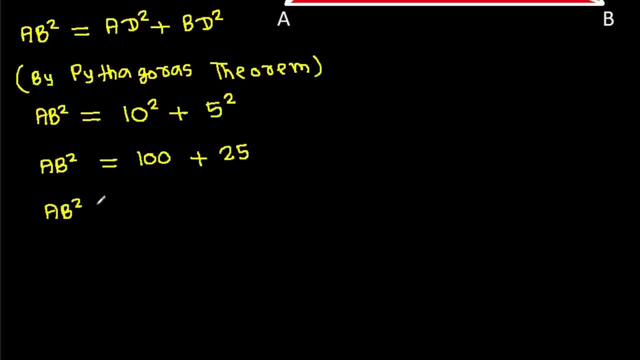 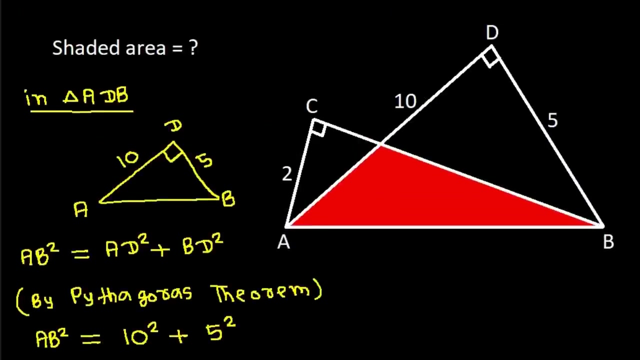 And AB squared it is 125.. So AB it will be equal to a square root of 125. That will be 5 times A square root of 5.. So we get AB: it is 5 times a square root of 5.. 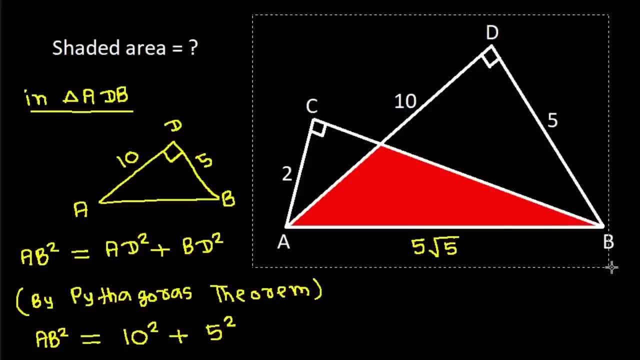 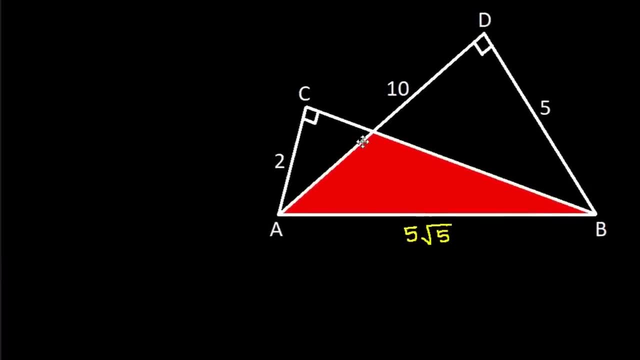 And And Now. So now we have to find embedded area. The correct answer is A, B and the P angle is 90 degree, and it is here that isшие new angle, this angle. The correct answer is A. And we have to find embedded area also like A, B and it is A, So we have to connect Hunter angle is 90 degree. angle AC is 1, and goes to composed angle is equal to 90 degree. 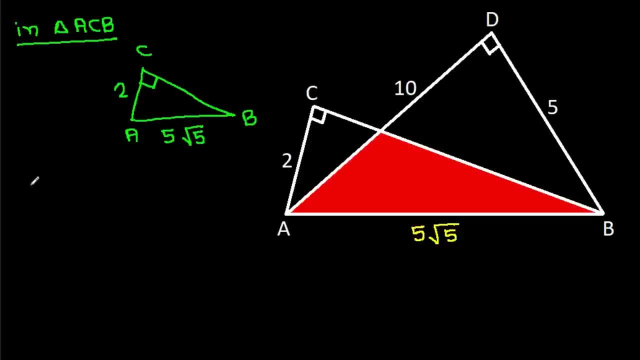 We have to find the other angle And this angle, isaire angle, is 5 times AP and you can calculate against this angle. These supports and oppose are the wind vitamin. So enter angle ACB, a, b square. it will be equal to a- c square plus b? c square by Pythagoras theorem and 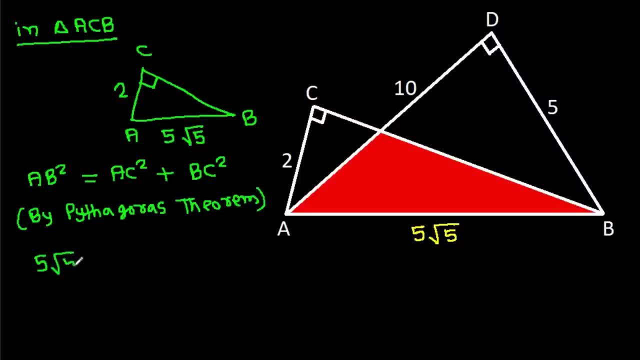 a b is 5 times a square root of 5 square. it is equal to a. c is 2 square plus b c square, and it will be 125 is equal to 4 plus b c square, so b- c square, it will be equal to 125. 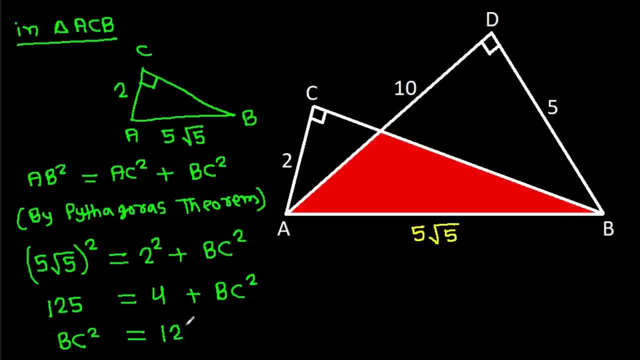 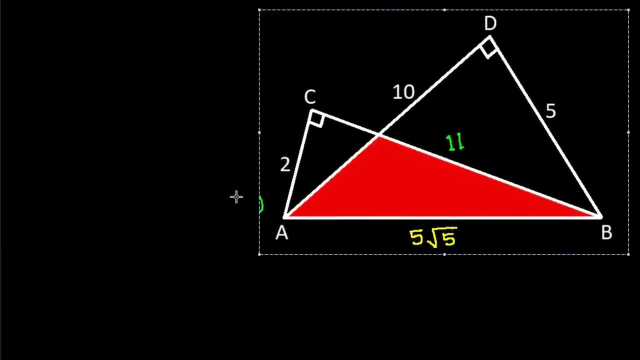 minus 4 will be 121, that means b c. it will be a square root of 121, that will be 11. so b c it is 11, and so b c it is 11. and Now we know that opposite angles they are equal. so here, suppose this point is E. then 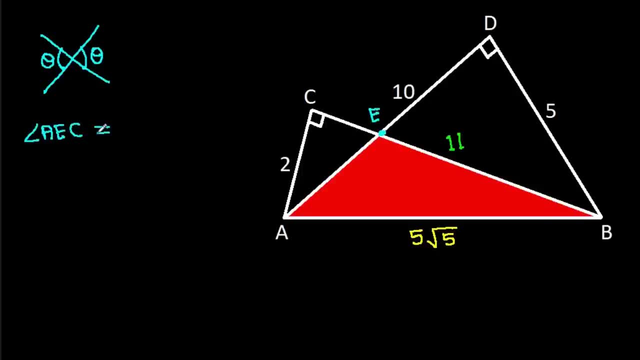 angle AEC it will be equal to angle BED. suppose theta these two angles, they will be equal. and now inter angle AEC and inter angle BED. we have: angle AEC is equal to angle BED, that is theta, and angle ACE it is equal to angle BDE, that is 90 degree. 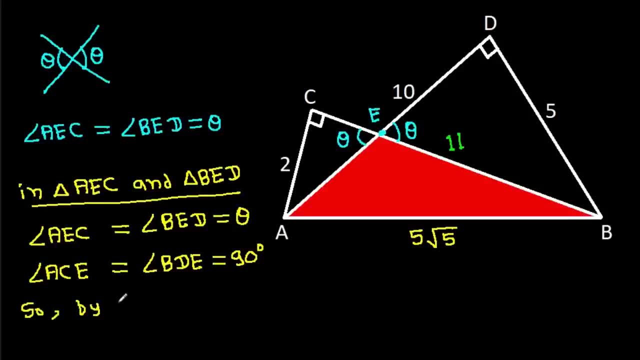 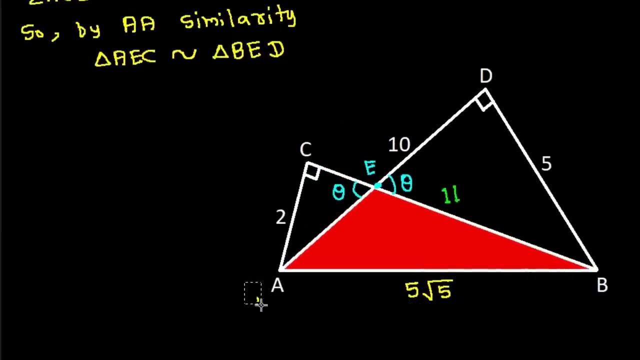 so by angle angle similarity, inter angle AEC- it will be similar to inter angle BED and These two are similar, Hence area of AEC. by area of BED it will be equal to AC by BD a square, and AC is 2 by BD is 5 a square, that will be 4 by 25.. That means if area of AEC is 4a, 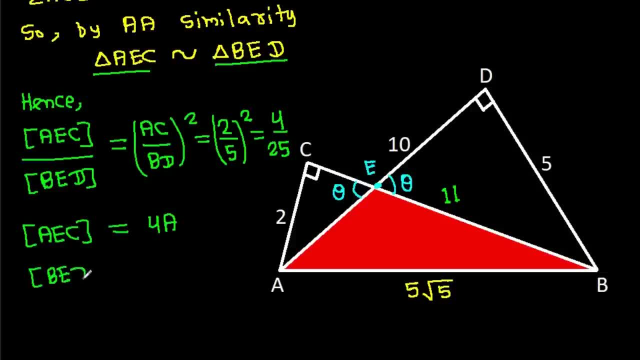 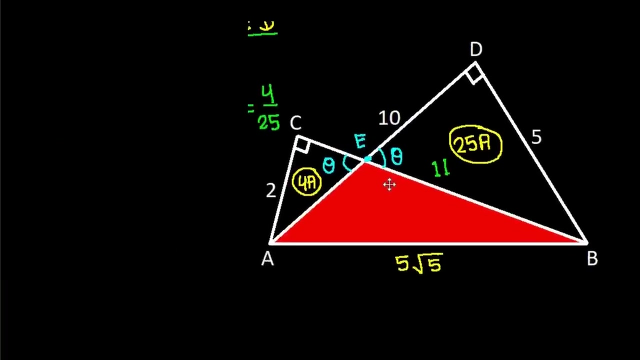 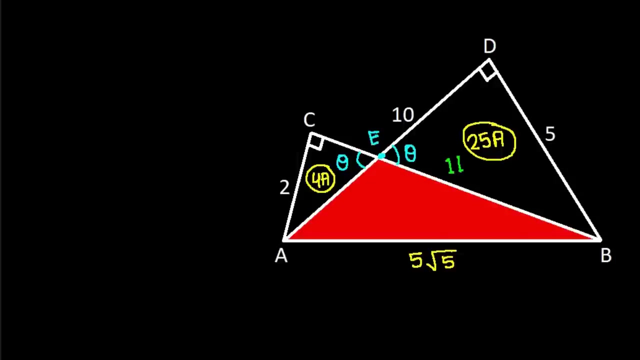 then area of BED, it will be 25a. If this area is 4a, then this area, it will be 25a. and now suppose area of AEB is x, this area is x. and now inter angle: ACB. it is ACB, this angle. 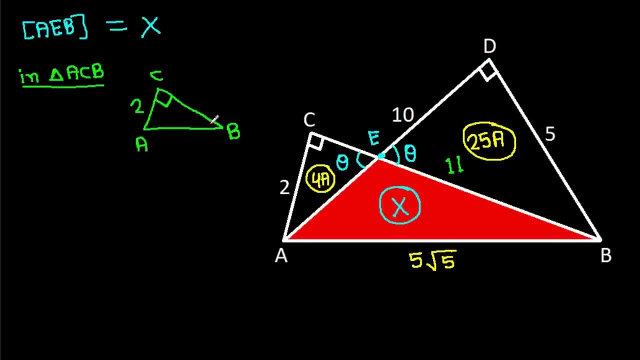 is 90 degree, AC is 2, BC is 11.. So area of ACB it will be 1 by 2 times base is AC and height is BC, and area of ACB it will be 4a plus x. It is 4a plus x, that is 1 by 2 times base is. 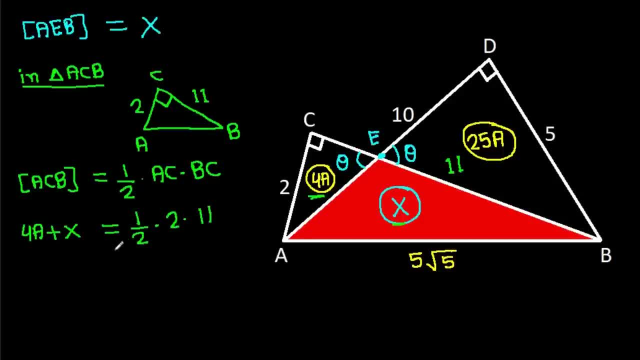 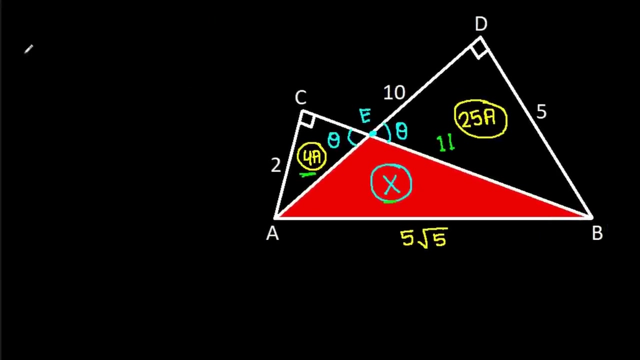 times ac is 2, bc is 11 and 2 will get cancelled. So 4a plus x it is 11.. Suppose it is equation 1 and inter angle adb. it is adb. this angle is 90 degree, ad is 10, bd is 5,. 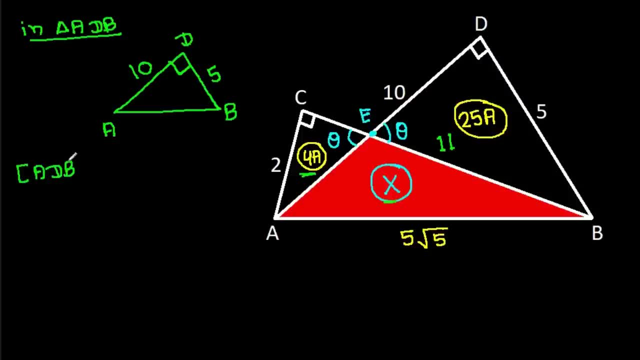 so area of adb it will be 1 by 2 times base is bd and height is ad, and area of adb it will be x plus 25a. it is x plus 25a. that is equal to 1 by 2 times bd is 5,. 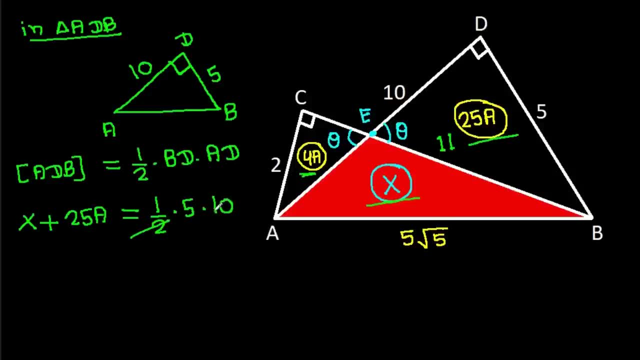 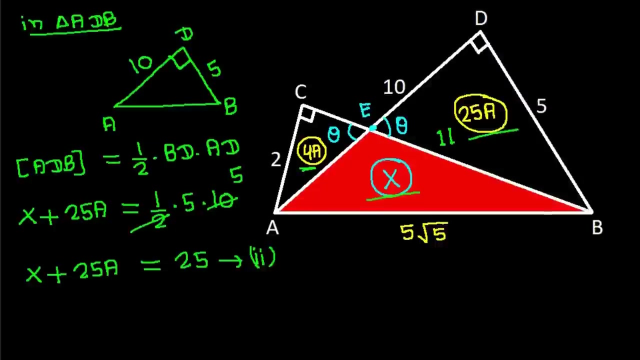 and ad is 10 and 2 times 5 is 10, so we get x plus 25a is 25.. Suppose it is equation 2, so we have 4a plus x is 11,. we have 4a plus x is. 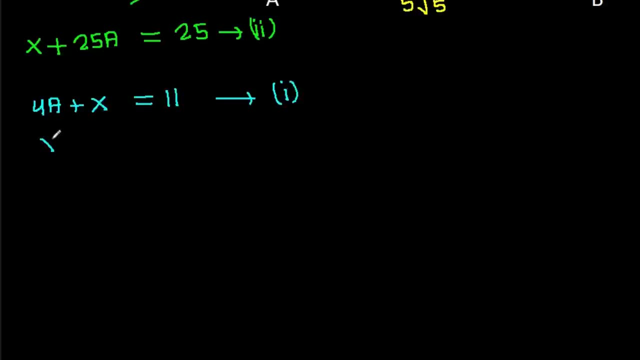 is 11, it is equation 1, and x plus 25a it is 25,, it is equation 2, and if we subtract equation 1 from equation 2, equation 2 minus equation 1, then x plus 25a minus 4a plus. 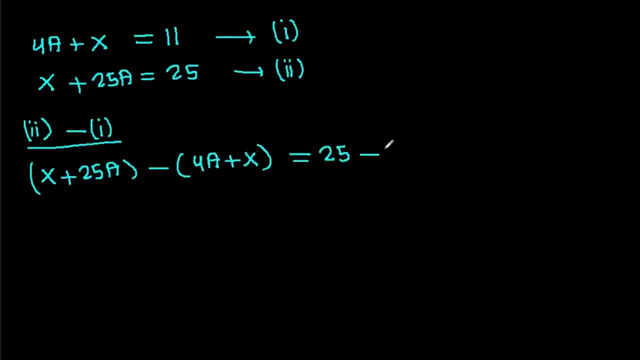 x, it will be 25 minus 11, and x will get cancelled. so 25a minus 4a it is 25, and 14, and 21a is 14,. so a it will be 14 by 21,, and 7 times 2 is 14,, 7 times 3 is 21,. so